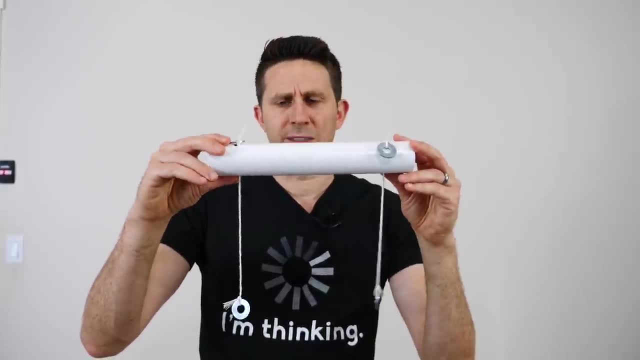 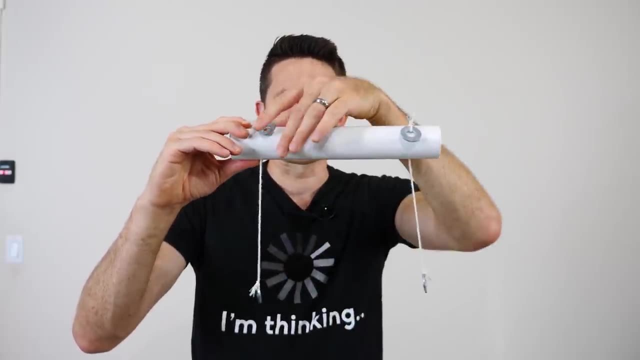 what we've observed in the past. So now, based on what we've observed, if I were to ask you what's going to happen when I pull this top string here, you'd probably say that it's going to make the bottom string shorter. So let's check and see if that's true anymore. 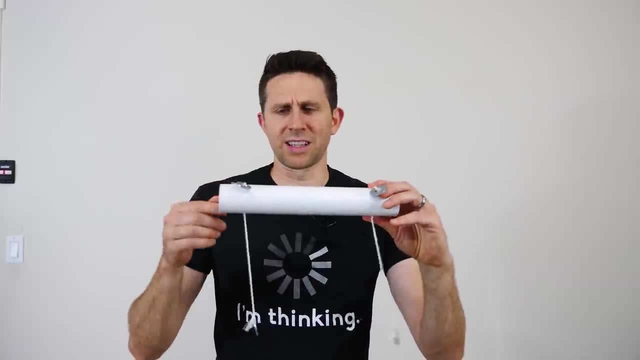 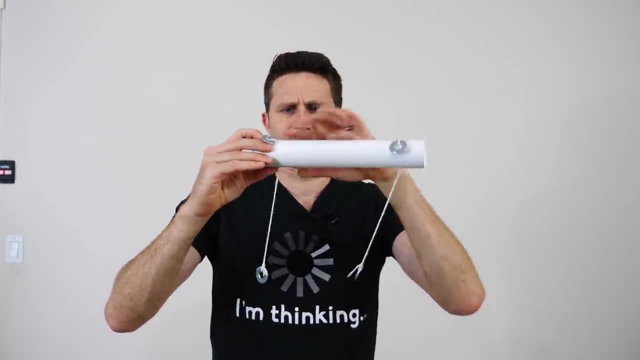 Suddenly. that's not true. So, based on what we saw, initially we might have assumed that when you pull the top one, the bottom one's for sure going to move up. But then suddenly, sometimes when you pull this one, it doesn't make the bottom one move up, but it makes this. 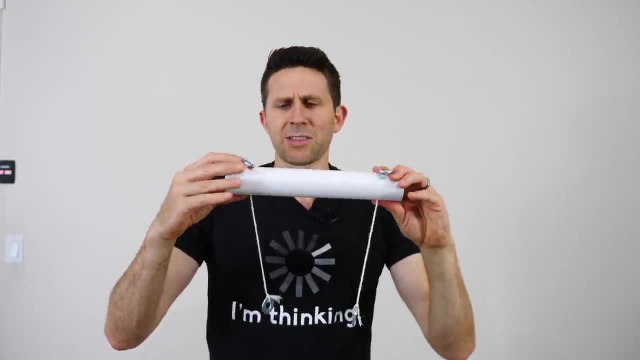 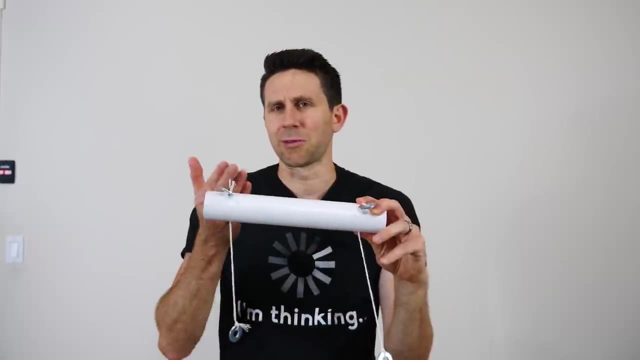 one move up, So we'd have to assume that there's something else going on besides what we initially guessed. what was going on? There must be some hidden variable that we're not understanding here. We initially thought we had it all figured out, that it was just a straight string going. 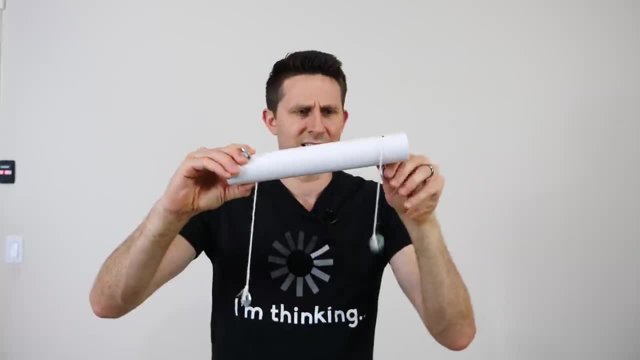 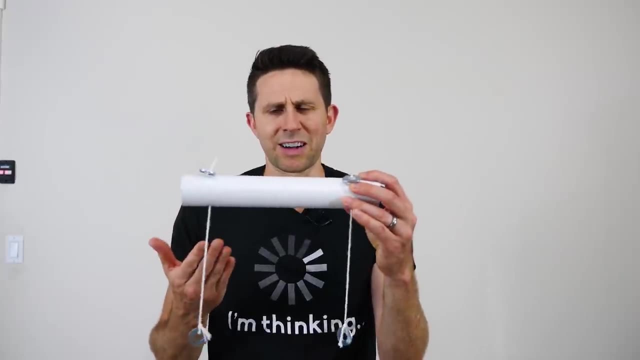 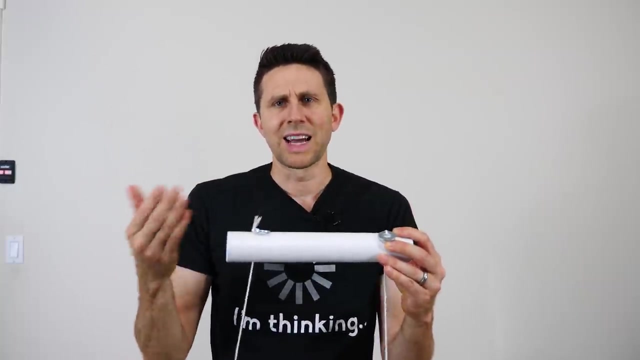 through. but it's obvious that that's not the case And we know there must be some hidden variable. because if this were true, that it were just randomly happening, what side of the string went up when I pulled this side? then that would mean that nature isn't deterministic. 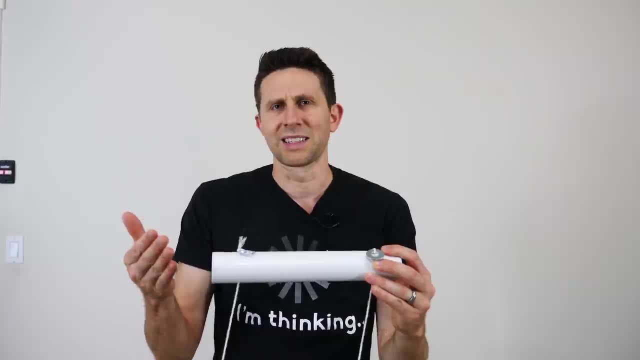 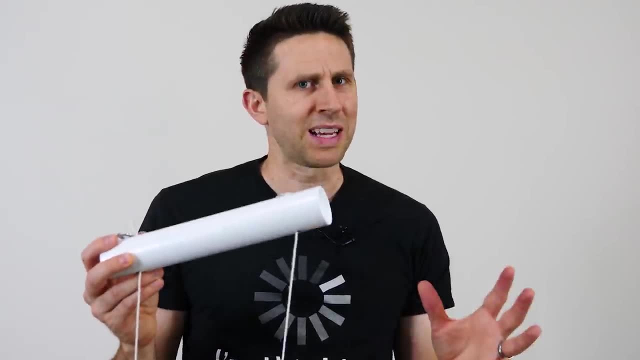 It would mean that nature is just random doing random things, And we don't like to build scientific principles based on randomness, But that's what quantum mechanics is based on. So let's see if we can actually figure out the hidden variable here. What's really going on here is that the strings 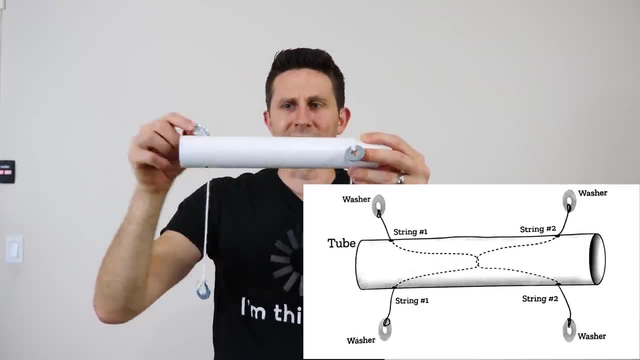 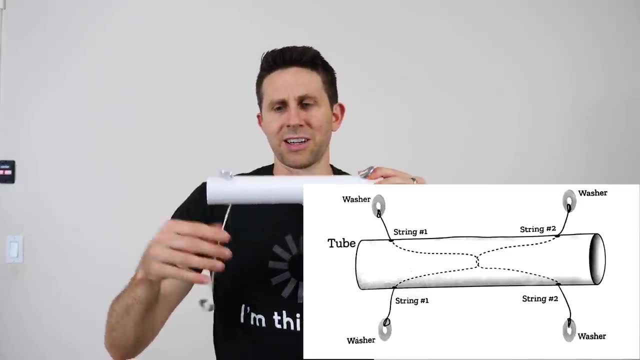 that are attached through here are actually wrapped around each other in the center, And so, depending on which of these holes you hold with your finger, you can cause one string to go up versus the other. They're all pulling on each other and they can slide past each other. 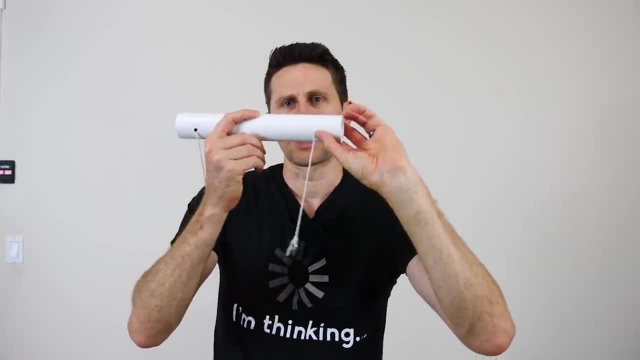 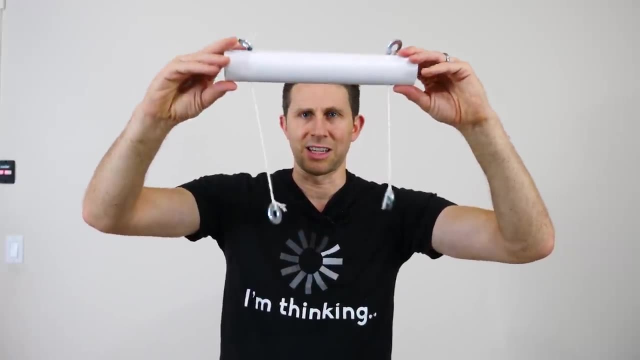 based on if I'm holding the string on the back here, You can see that I'm actually covering the hole with my finger, And so that causes this side to go up and down. But if I don't cover that hole and cover the other side, 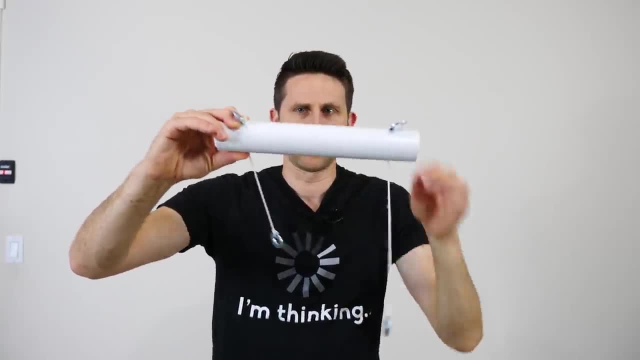 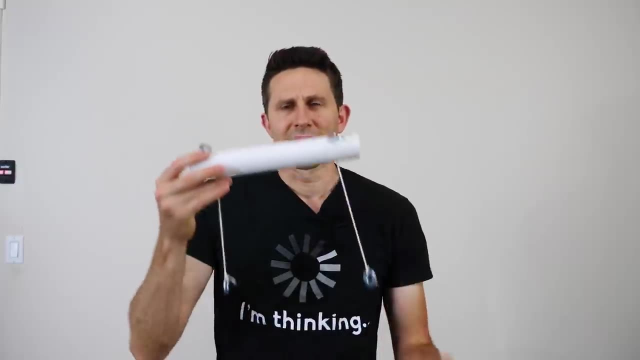 then it's gonna let this one be able to move. So the true hidden variable was that in the center the strings are wrapped around each other, And so it causes it to look like there's some random thing happening, when really it was just a simple mechanism inside. 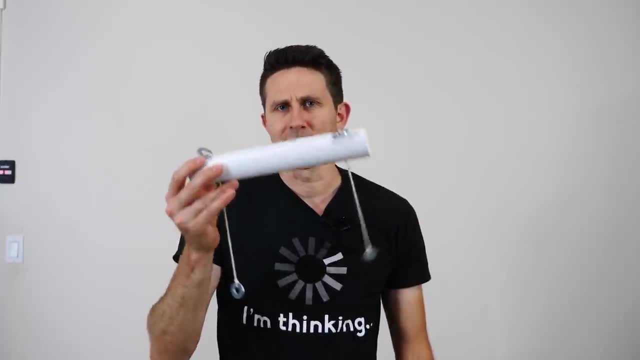 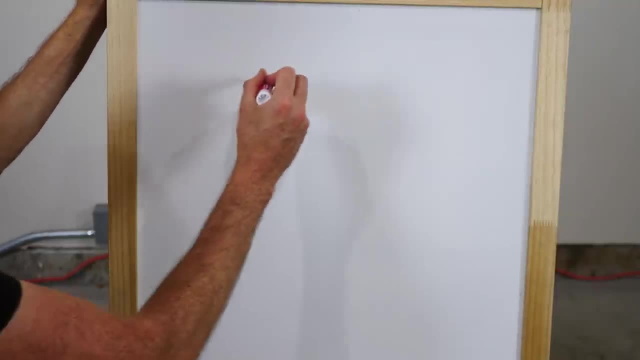 that we couldn't see. So that was the true hidden variable that we were missing in order to make an accurate scientific prediction. So now let's compare this to an experiment in real life, like measuring the spin of an electron. Whenever you measure the spin of a single electron. 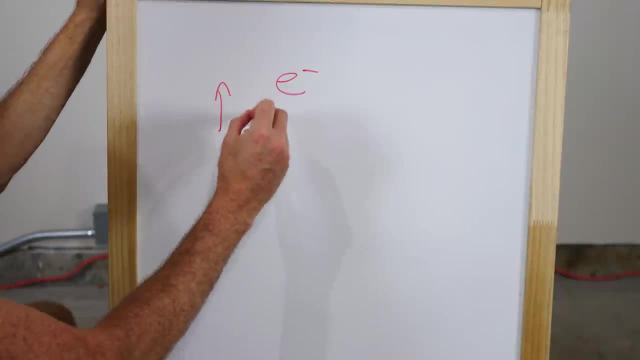 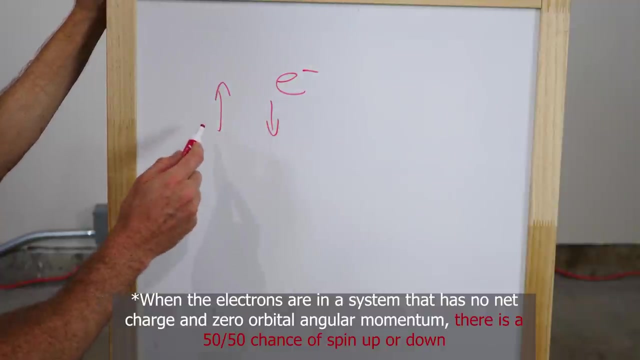 you'll find that it's in one of two states, either spin up or spin down. And it turns out we've found absolutely no way to know beforehand what state that electron's going to be in before we measure it. There's no possible prediction we could make. 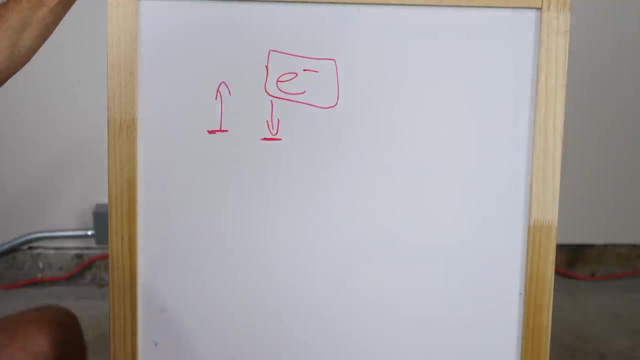 to know for sure what it's going to be, But, just like in our tube string experiment, you may be too going to be able to measure the spin of a single electron, And you may be tempted to say that we're just missing something. 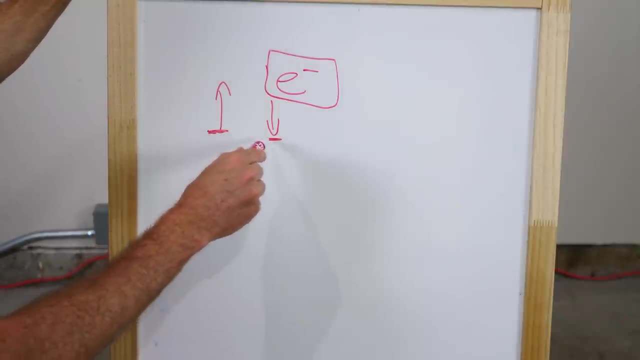 There must be some hidden variable here that's causing it to be either spin up or spin down before we measure it. but we only know what it is once we measure it And it turns out, if you're thinking, that you're in good company. 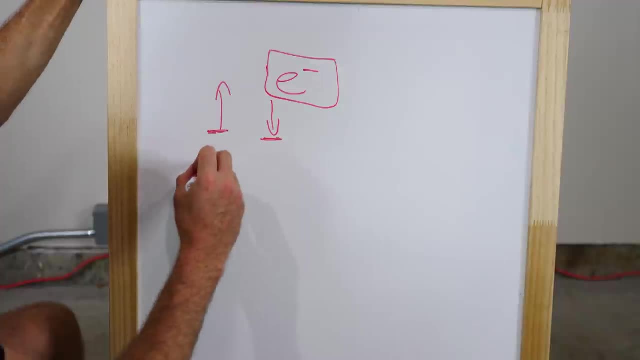 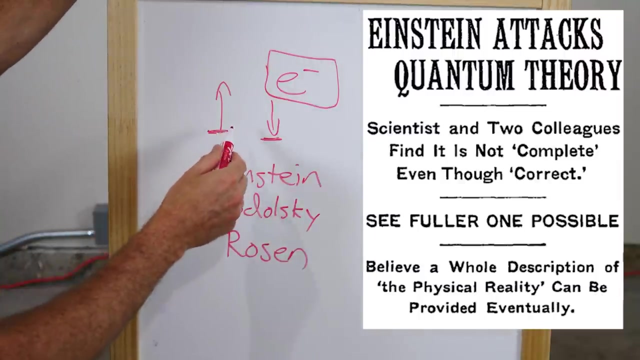 because, when quantum mechanics was just beginning, three physicists- Einstein, Podolsky and Rosen- argued that there must be some hidden variable and thus quantum mechanics is not a complete theory, And this became known as the EPR paradox. They showed that, due to the randomness of quantum mechanics, 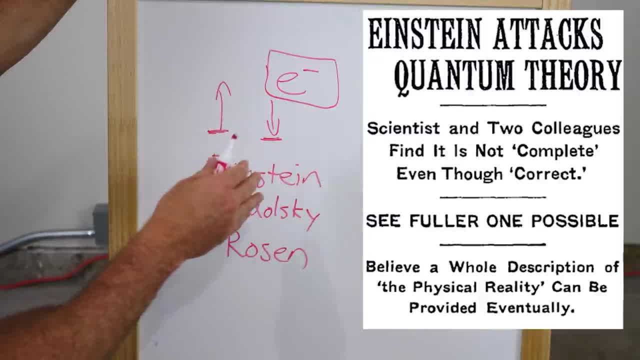 quantum mechanics breaks locality, meaning that it doesn't follow special relativity, And so these physicists argued that there must be something that we're missing. They argued that there has to be some hidden variable that we're not noticing. However, later, a physicist named John Bell 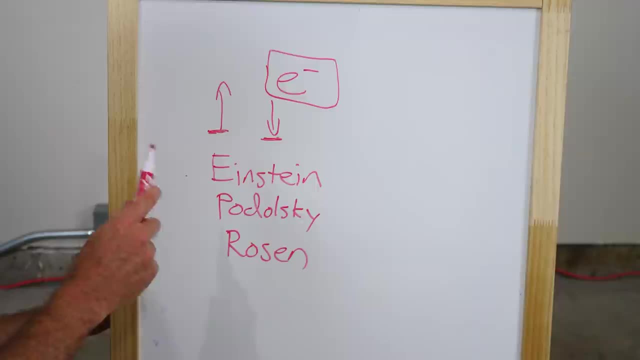 came up for a solution to the EPR paradox, And John Bell showed that it's not possible that there are hidden variables in quantum mechanics, And this became known as Bell's law- Bell's theorem. Now let me explain what Bell's theorem is. 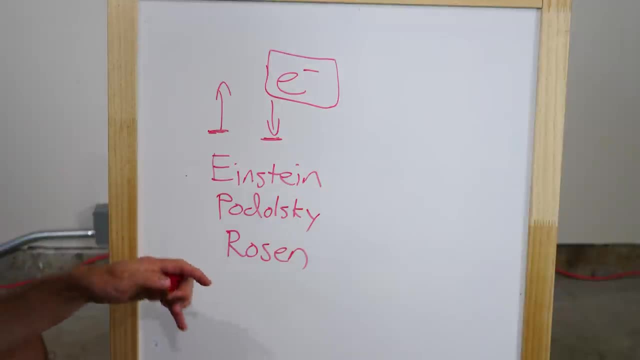 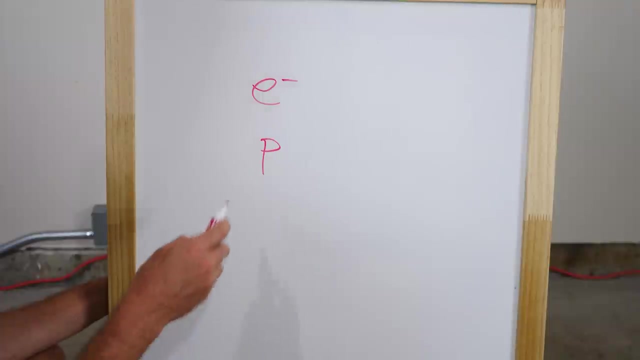 and how we know for sure that there's no hidden variables in quantum mechanics. Now, instead of using an electron to prove Bell's theorem, I'm gonna be using a photon instead. Now, photons can be either vertically polarized or horizontally polarized, And just like our randomness of the electron, 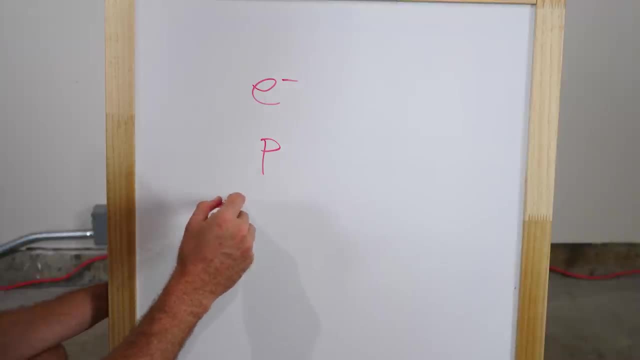 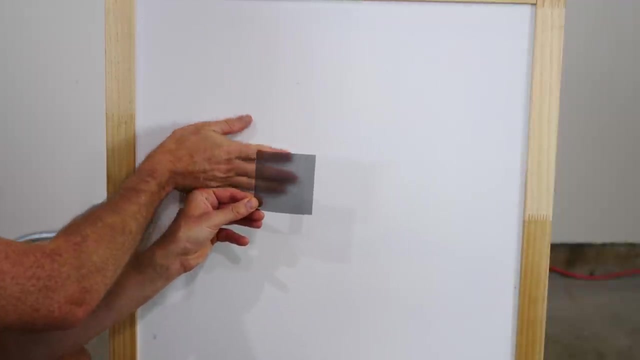 it's not known beforehand, when we measure a photon whether it's gonna be vertically or horizontally polarized. For example, I'm gonna take this polarizer here and you can see that it exactly diminishes the light coming off of this board by 50%. 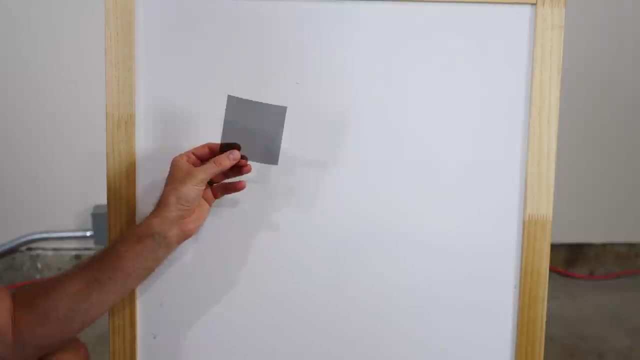 So 50% of the light coming through this was vertically polarized. It turns out that when you take another vertically polarized filter and you turn it at a 45 degree angle to it, it then will let through 50% of that original light. 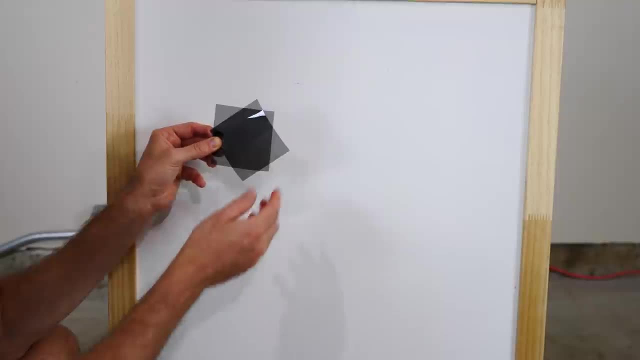 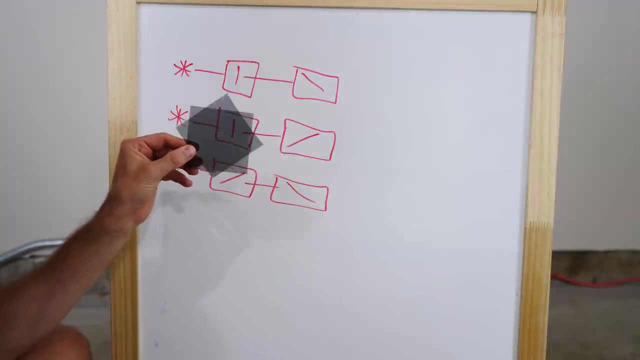 So 50% of the light that came through this polarizer is now coming through this one. So in this first case, if I take a vertical polarizer and a polarizer that's turned at 45 degrees to that, you'll see that I get about 50% of the light coming through. 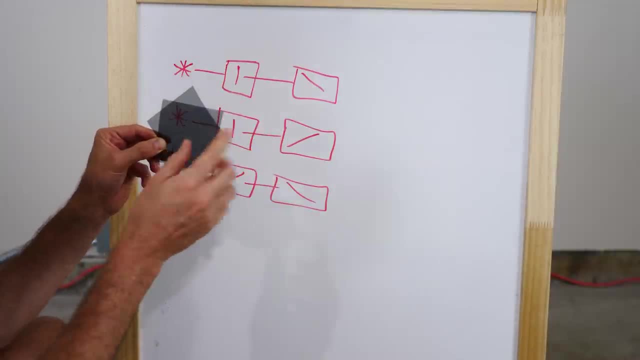 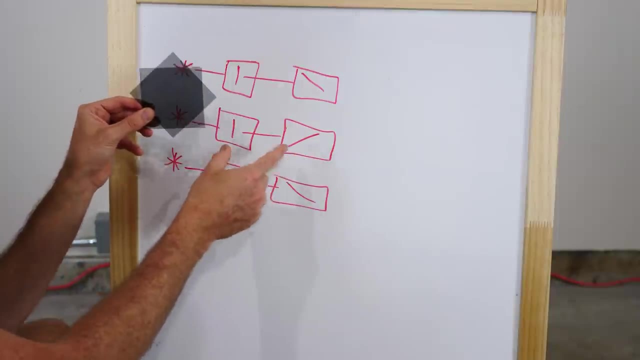 So about 50% of the photons that made it through this first one also make it through the second one, And if I take one that's turned the opposite direction, I get the same results when I put them together: About 50% of the photons. 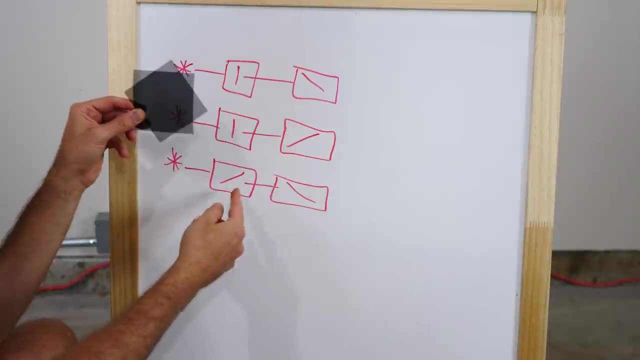 that made it through this first polarizer, make it through the second one. But now if I take a 45 degree polarizer turned in this plus 45 degree, I get about 50% of the light coming through. And if I take one that's turned in the negative 45 degrees, 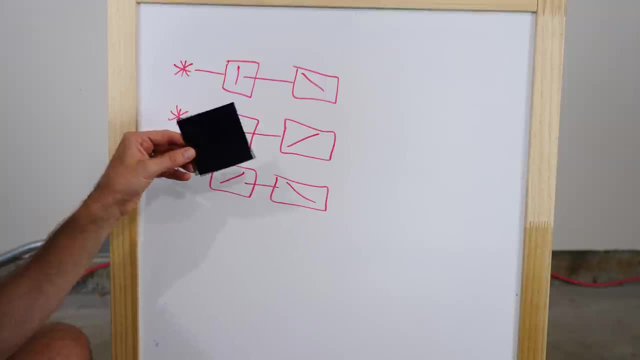 and then one turned in the negative 45 degrees, you'll see that I get no light coming through. So this completely blocks the light. If you look at this on an individual photon case, instead of just sending through a bunch of light like I'm doing here, 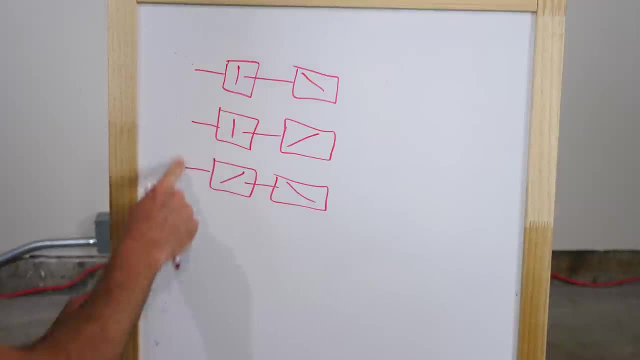 let's just send through one photon at a time, But the thing is we don't know the polarization before we measure it. So if I send through only one photon, there is a chance that I'm gonna measure it on the other side. 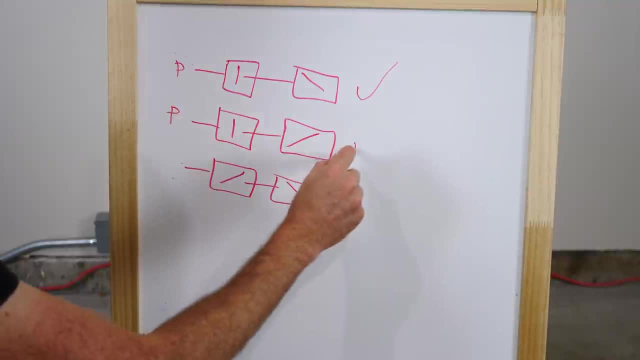 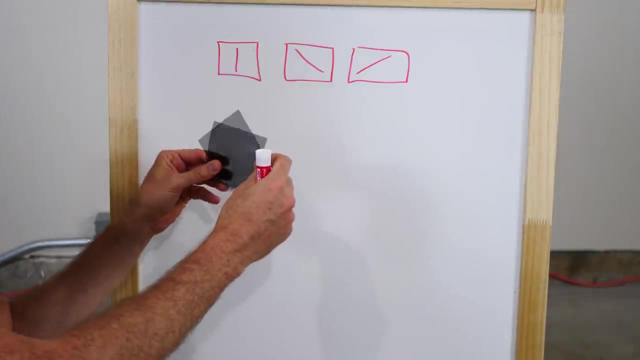 So I'm gonna say: this has a chance, This one also has a chance, But this one has no chance of getting through. So in this experiment, the chance of being able to measure one single photon is completely random and unpredictable in quantum mechanics. 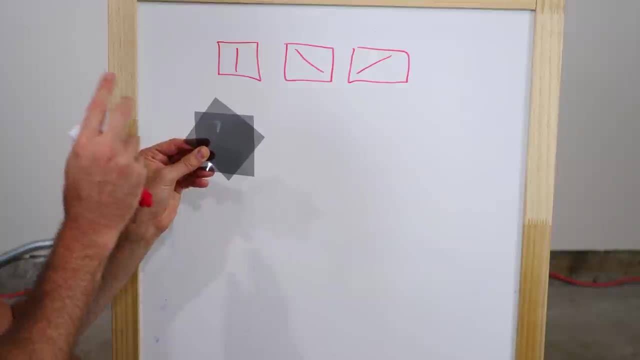 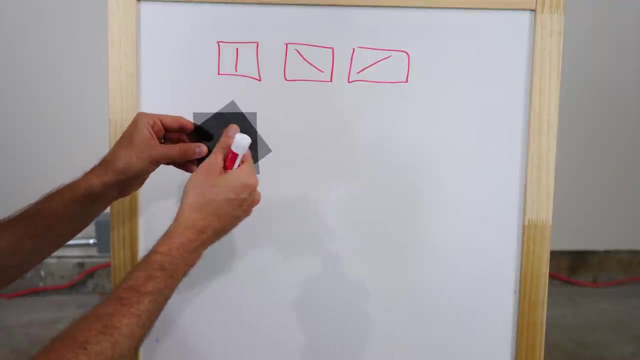 We know the probability for one single photon, but we can never know for sure the chance of seeing that photon come through. We know that any photon that makes it through this one only has a 50-50 chance of making it through this one. 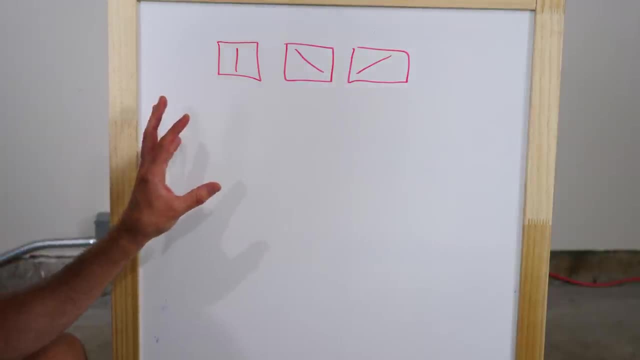 But you might say there's actually some hidden variable that we're not accounting for. A picture can't just be random like that. We have to be able to predict it somehow. We just don't understand it completely. So let's say that were the case. 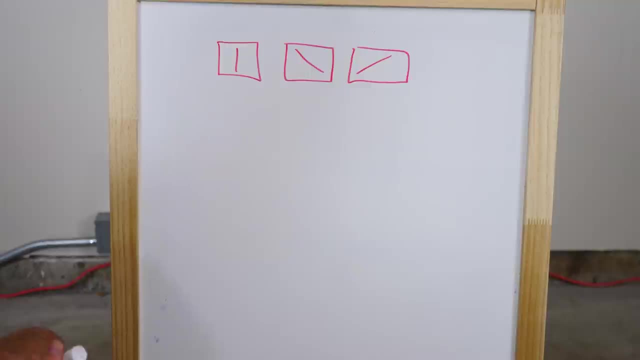 If that were the case, then we'd have to say that there's some hidden variable that tells it beforehand whether or not it can make it through a polarizer angled like this, a polarizer angled like this, or a polarizer angled like this. 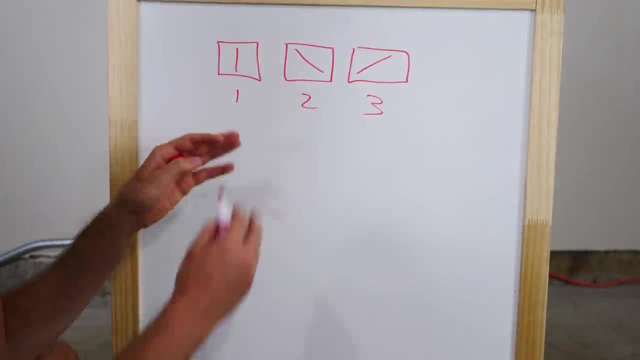 And let's just call these options one, two and three. So let's just say there's some hidden variable that we don't know, that somehow has this information contained in it and it's a photon that's predetermining whether it can make it through. one, two and three. 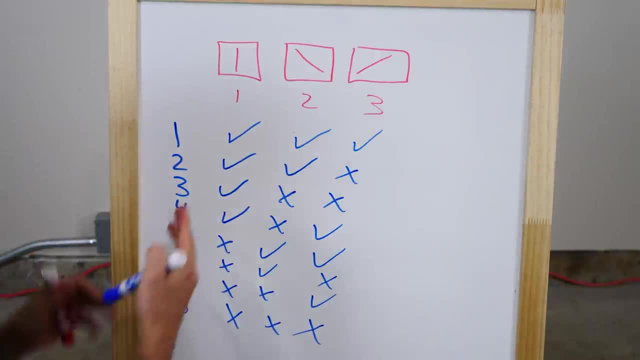 Well, even though we don't know what the hidden variable is, we can try to know something about the hidden variable if it existed. There's only eight different pieces of information that that hidden variable could have. It could have the information that the photon 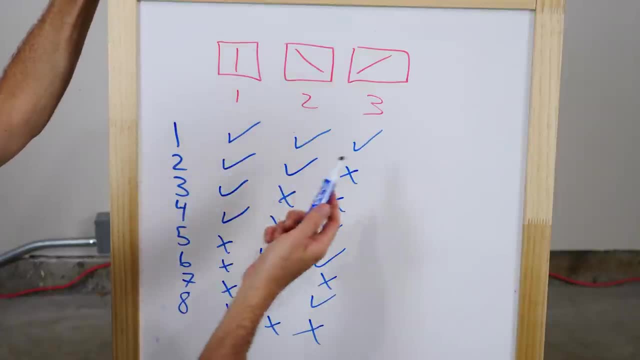 can make it through polarizer one, two and three. It could have the information that it could only make it through one and two, but not three. It could have the information that it can only make it through one and not two or three. 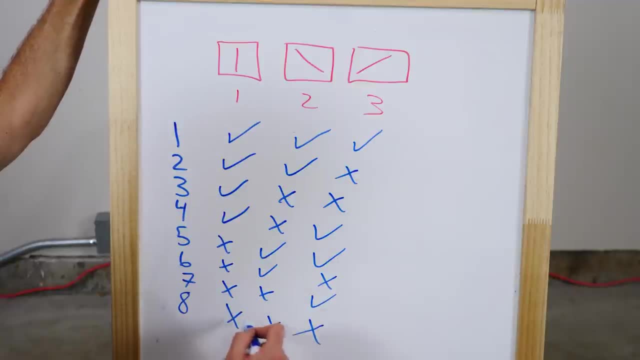 and so on until number eight, where it has the information that it can't make it through any of them. So these are the only bits of information that it can have. So the hidden variable would have to have one of these options tattooed on it beforehand. 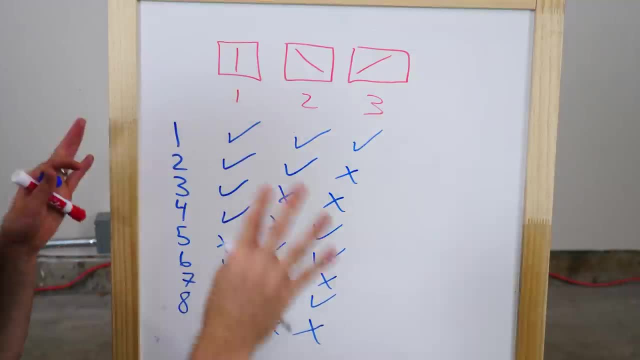 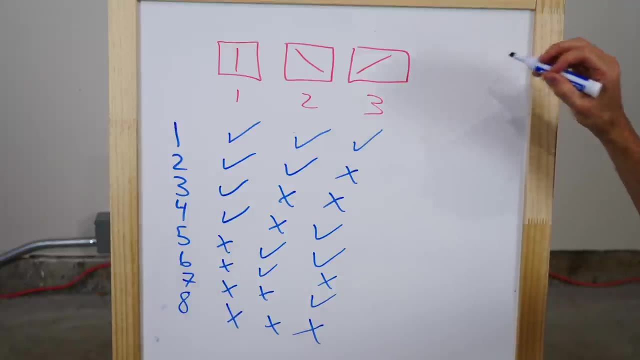 and so it knows whether it can go through each of these beforehand. And it's not random, it's a hidden variable. Now, with this information, we're going to do an experiment. In this experiment, we're going to be using entangled photons. 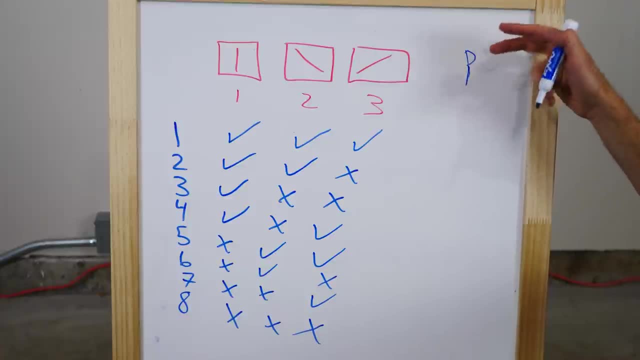 Entangled photons means that you have a pair of photons that, whatever you measure the polarization in one of them, the other one is for sure going to have, And these exist in real life. So that means, if you measured photon one, to have this vertical polarization. 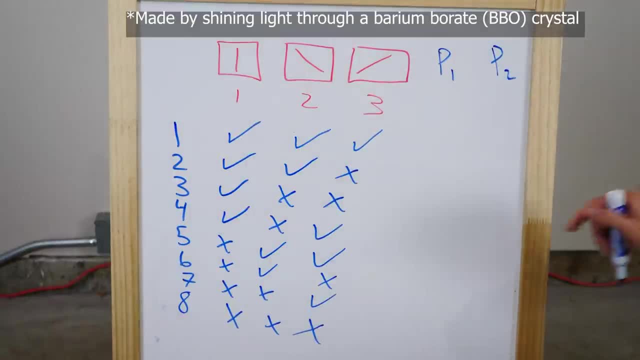 then for sure photon two is going to have that same polarization. And also, if you measured this photon to make it through this polarizer turned in the 45 degree angle, you'd know for sure that this photon's gonna be in that 45 degree angle. 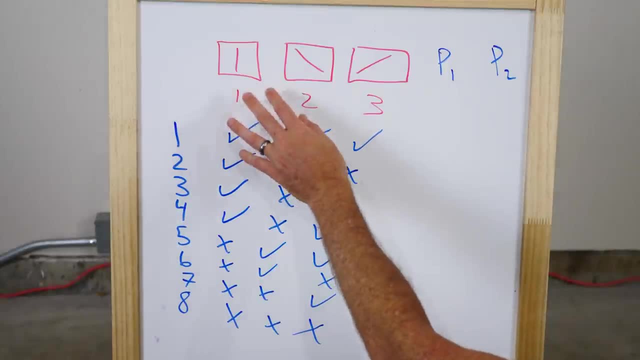 These are called entangled photons. Even though in each of these cases it's only a 50-50 chance whether this photon's gonna make it through or not, you do know that when it comes through, this one will for sure also make it through. 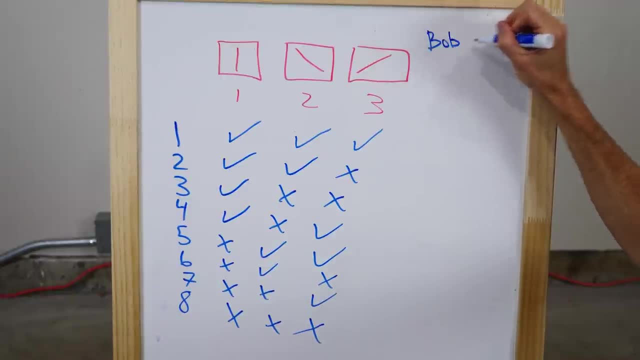 So in this experiment we're going to be shooting these entangled photons at two people. I'm gonna call them Bob and Sue. We're going to shoot these entangled photons at Bob and Sue. One goes to Bob, the other goes to Sue. 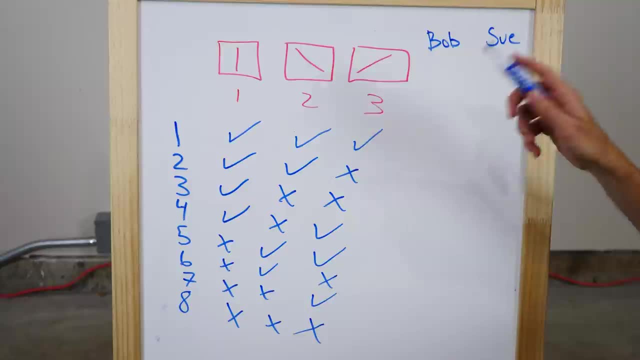 And they're going to randomly grab one of these polarizers and just measure whether or not the photon came through. So what we're gonna do is we're just gonna record whether or not Bob and Sue got the same results. Whether or not it came through or not doesn't matter. 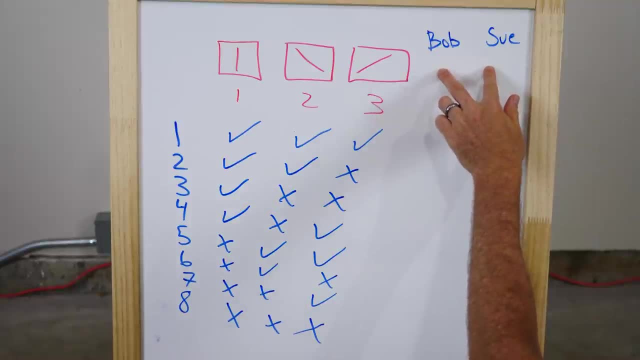 We're just gonna say they got the same results or they didn't. So either they both saw a photon come through or neither of them saw a photon come through. So if the photon's polarization were predetermined, we already wrote down what that predetermined information. 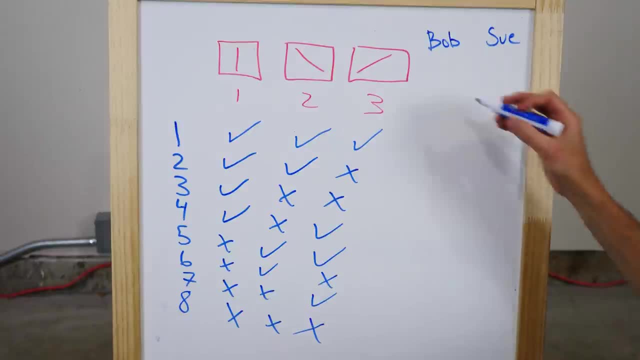 could be. So let's go through each of these probabilities. So in the first case, one of them could grab polarizer one and the other one could grab polarizer two. Or one of them could grab polarizer one and the other one could grab polarizer three. 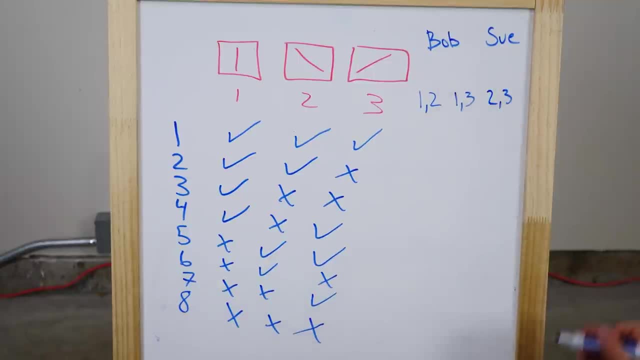 Or one of them could grab polarizer two and the other one grab polarizer three. And now we're gonna look at the possibilities of these hidden variables and see what the results would be if there were these hidden variables. So if the hidden variables were that, it should have gone. 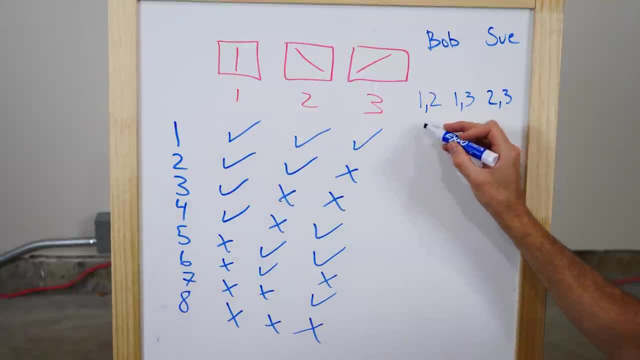 through one and two. we can see that it went through one, went through two, so they're gonna get the same results. And also one and three. they're gonna get the same results. And two and three: they're gonna get the same results. 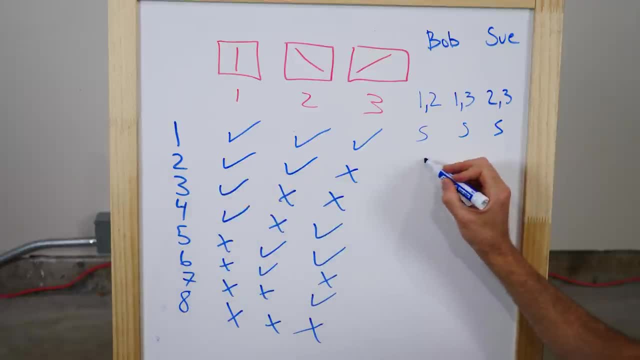 But if the hidden variable were number two here, then we're gonna say: one and two have the same results, One and three don't have the same results, so that's different. And two and three don't have the same results, so that's different. 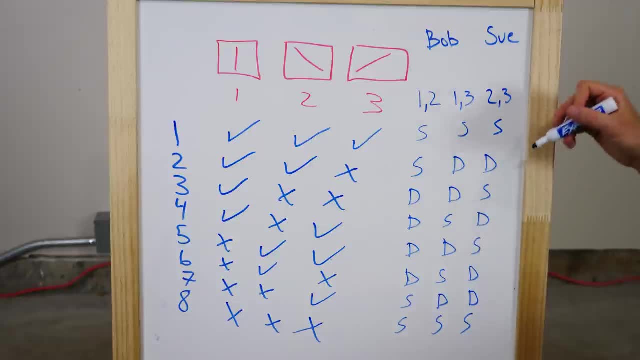 And if you go through all of these possible outcomes, you'll find that the lowest probability that could happen of having the same results is one third. In case number eight: there's 100% chance that you'd get the same results. In case number one: there's 100% chance. 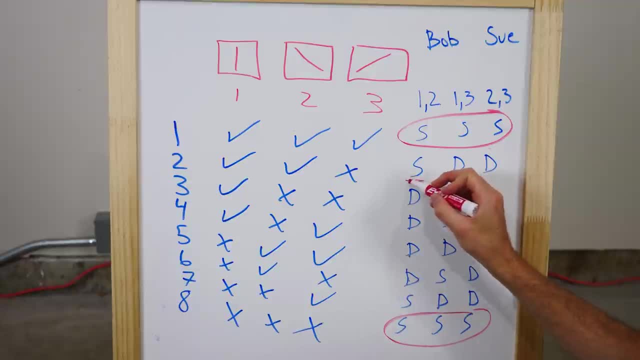 But if your hidden variable was number two here, there's a 33% chance- one out of three- that you would have got the same results, And that happens to be the case for all of the rest of the possibilities here. So for whatever the possibility of the hidden variable was, 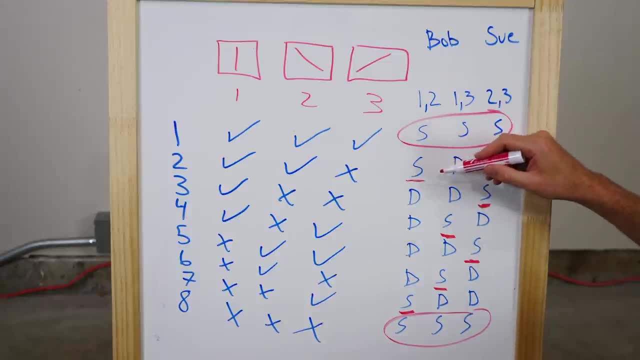 the lowest possible percentage you could get the same results is one third. So I'm just taking the lowest percentage out of each of these possibilities: 100%, 100%, and then each of these is 33%. So the lowest possibility in an experiment. 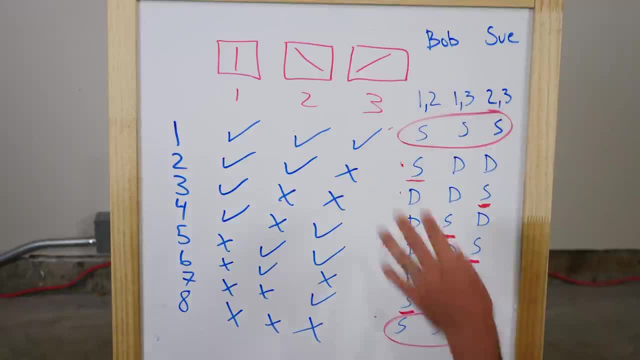 that you could get the same results should be 33% if there were these hidden variables here. So that means if you just set up this experiment in real life, if there are hidden variables because we drew out all the possibilities of any hidden variable would have to be. 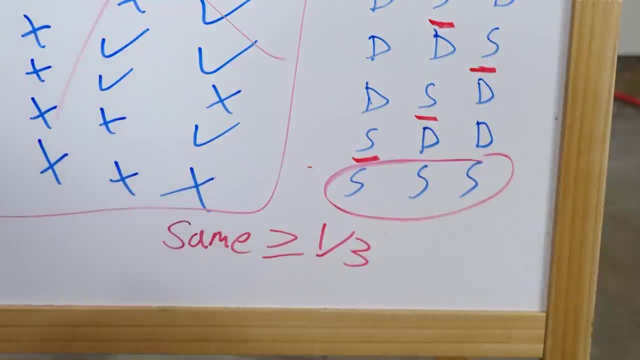 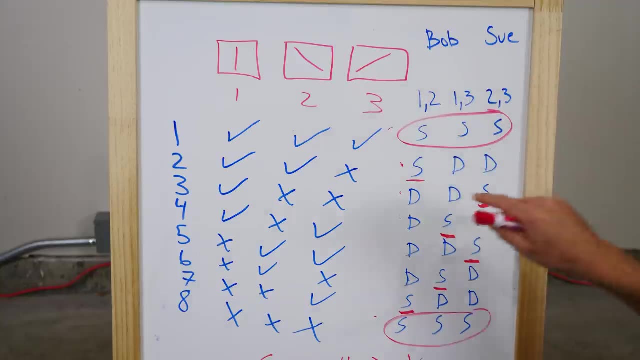 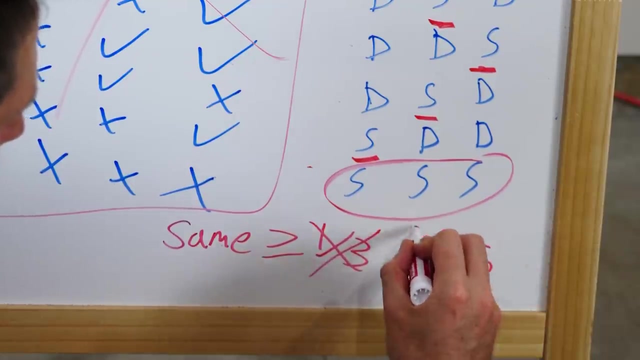 greater than or equal to one third. But it turns out, when you actually do this experiment and set up an entangled photon pair sent to two observers using polarizers like this, you don't get one third, You get only around 25%. 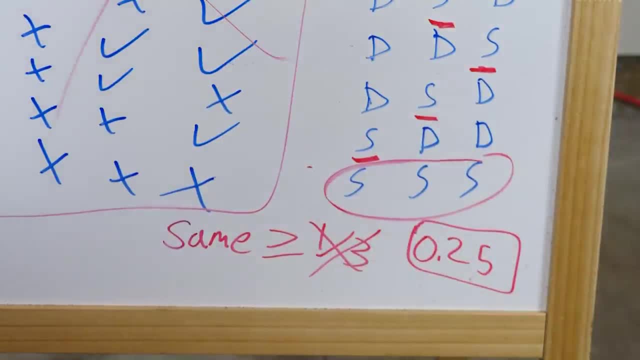 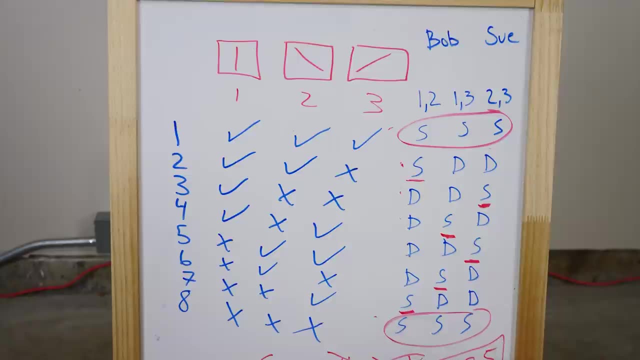 This is one application of Bell's theorem that proves that there can't be hidden variables in quantum mechanics. If there were hidden variables, we'd expect that when we actually do this experiment in real life, the lowest possible probability of them getting the same results is only around 33%. 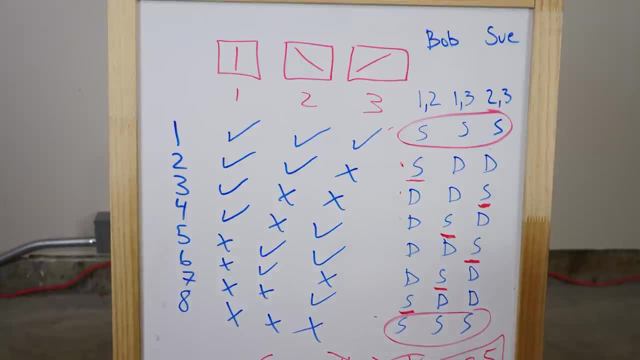 But it turns out when we do this experiment, it's only 25% chance that they get the same results. So what this means is that saying that there are these hidden variables that could assign a polarization state to a photon, but we just don't know what the hidden variable is. 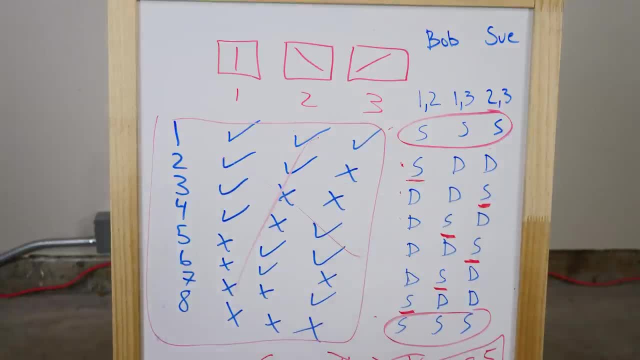 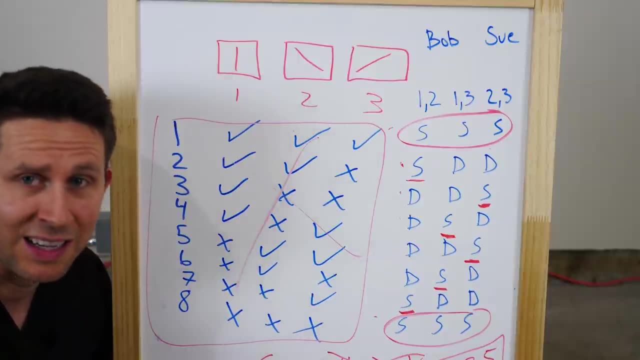 it means that this is not true. There are no hidden variables in quantum mechanics. It means that there truly is randomness in quantum mechanics, But it turns out that's not so bad. Even though randomness rules in quantum mechanics, you can make probability predictions. 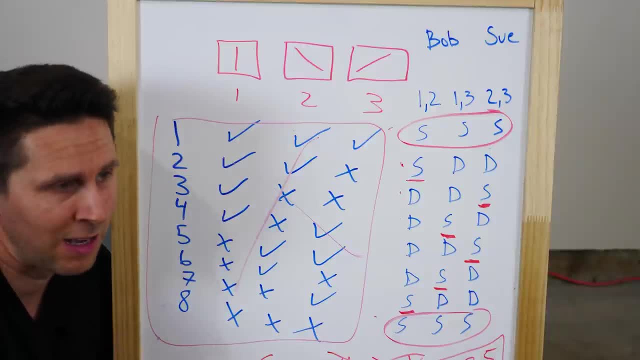 based on a lot of things happening. So we can still predict what will happen to a big group of things like 10 to the 26 atoms or electrons or photons, but we can't predict what one state will be in one photon or one electron. 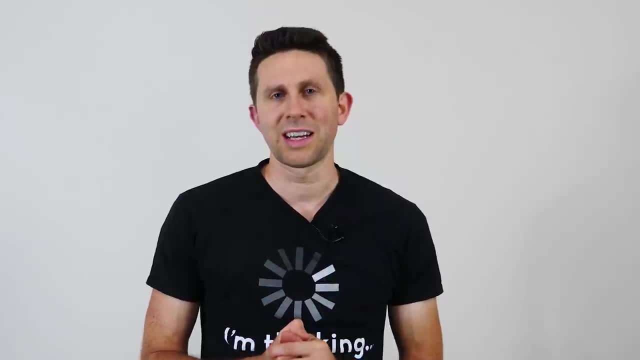 Hey everyone, thanks for watching another episode of the Action Lab. I hope you enjoyed it. If you did, don't forget to subscribe if you haven't yet, and also hit the bell so you can be notified when my latest video comes out. 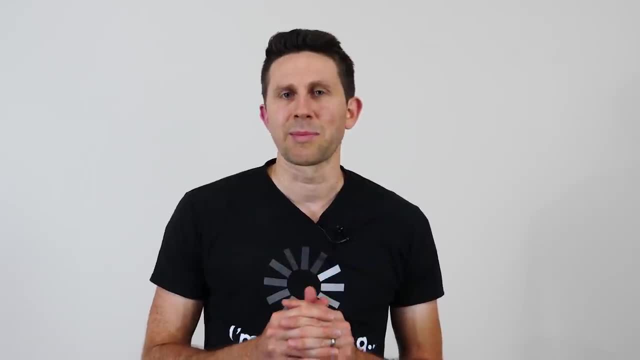 And check out theactionlabcom for the Action Lab experiment boxes if you haven't got yours yet. And thanks for watching and I'll see you next time. 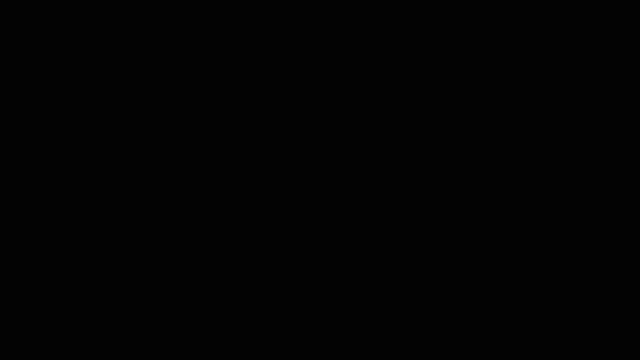 In this video we're going to talk about how to determine the maximum number of electrons given a certain set of quantum numbers. So let's say, if n is equal to 7, what is the maximum number of electrons that will have an n value of 7?? n is the principal quantum number, by the way. 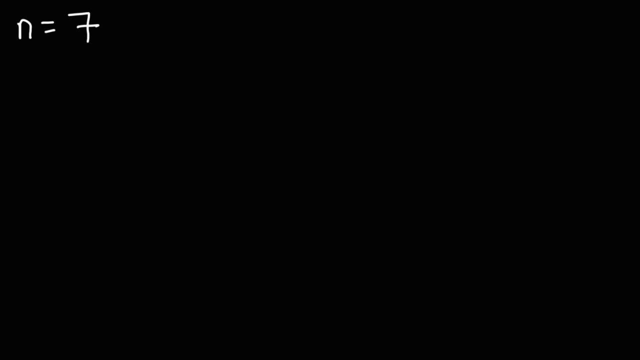 Well, there's a formula that we could use to get the answer. But first let's understand how to get the answer. When n is 1,, there's only one possible orbital that we can have, and it's the 1s orbital. s can hold a maximum of 2 electrons. Now, when n is 2,, 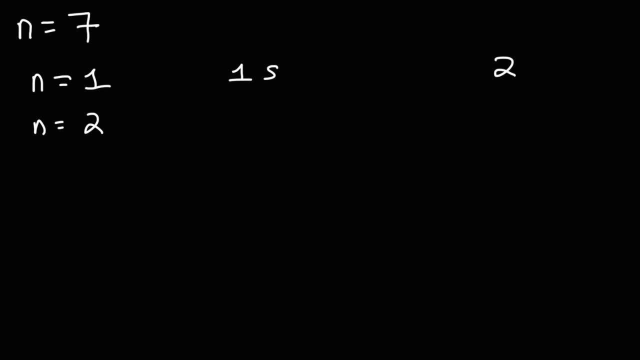 you could have the 2s orbital. Let me rewrite this here: You could have the 2s orbital and you could have the 2p orbital. p can hold up to 6, electrons s can hold up to 2.. 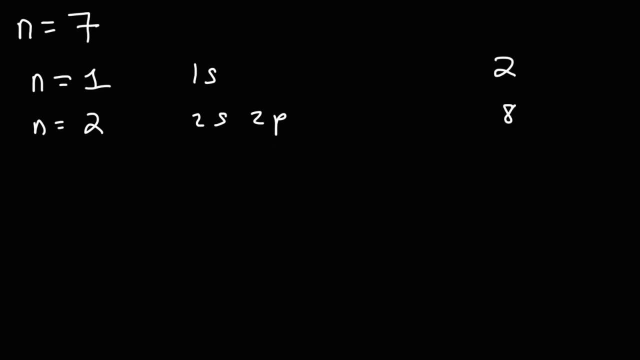 So you can get a maximum of 8 electrons in the second energy level. In the third energy level there are three sublevels: 3s, 3p and 3d. d can hold up to 10.. So if you add 8 plus 10, you get a maximum of 18 electrons in the third energy level. 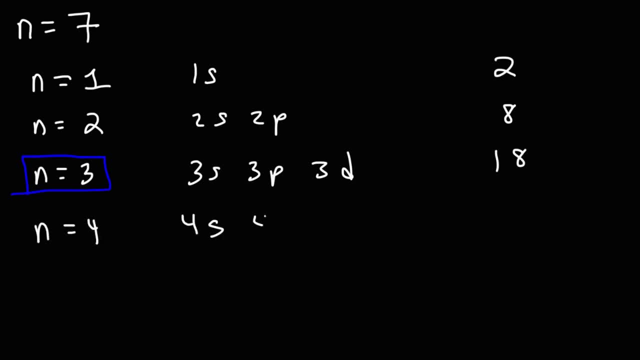 In the fourth energy level there are four sublevels: 4s, 4p, 4d and 4f f can hold up to 14 electrons. So if you add 18 plus 14, that gives you a maximum of 32 electrons. 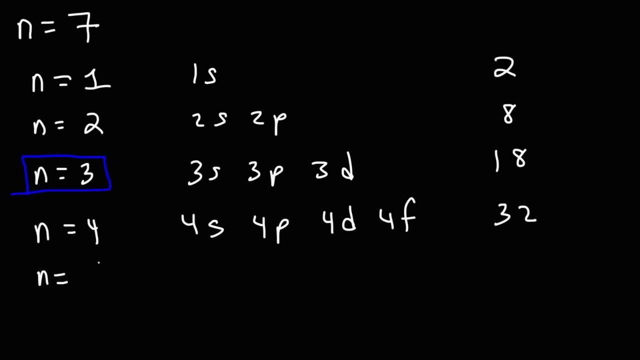 in the fourth energy level. Now for n equals 5, you have the 5s, 5p, 5d, 5f. I believe the next one is 5h or something, But whatever it is, it's going to be if s can hold up to 2,.